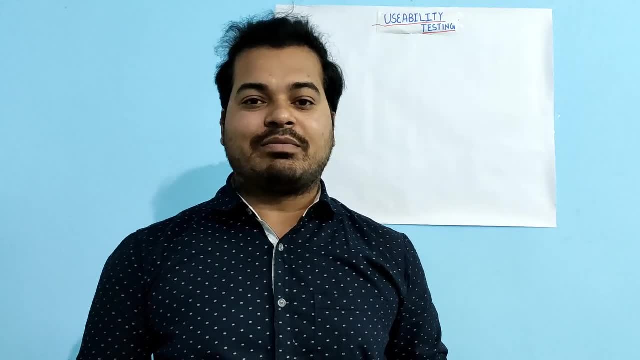 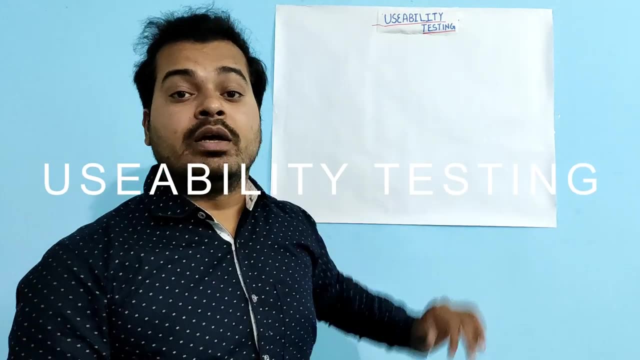 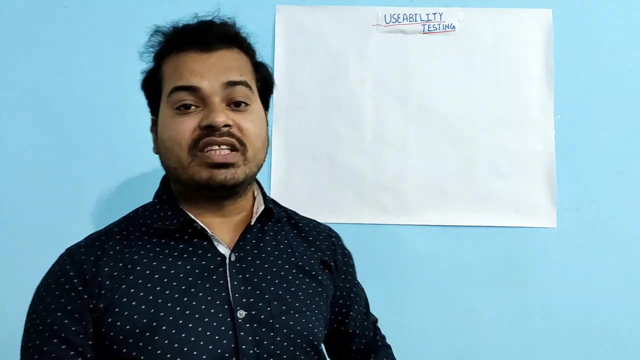 Hi, I welcome you all to my YouTube channel, Software Testing by NKT. In this video we are going to talk about. what do you mean by usability testing in software testing? Before we proceed with this video, make sure that you hit the subscribe button down below. Let's get started with the usability testing. 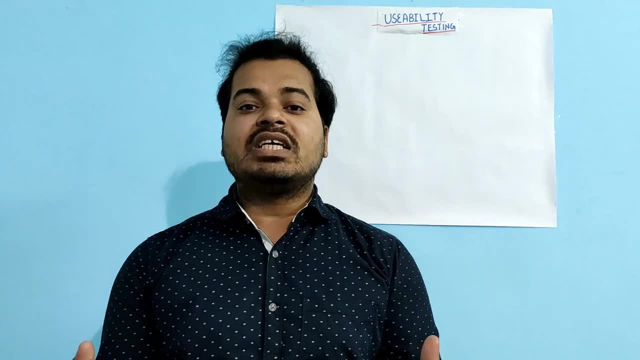 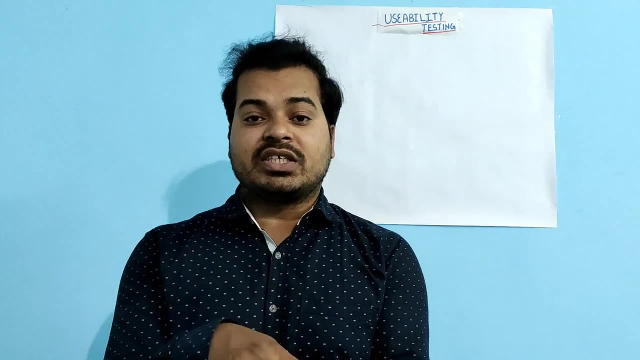 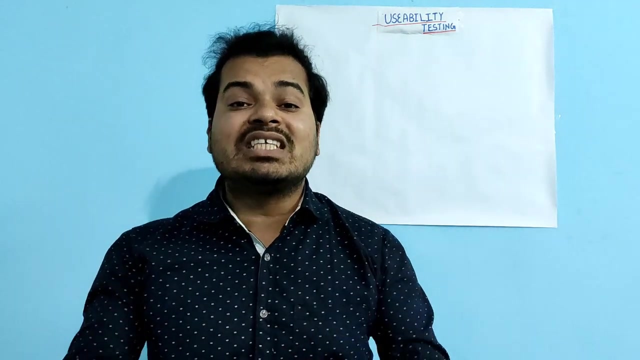 Usability testing is nothing but testing the user-friendliness of an application, How friendly it is to use that particular application for the user. that is called as usability testing. Testing the user-friendliness of an application is called as usability testing. 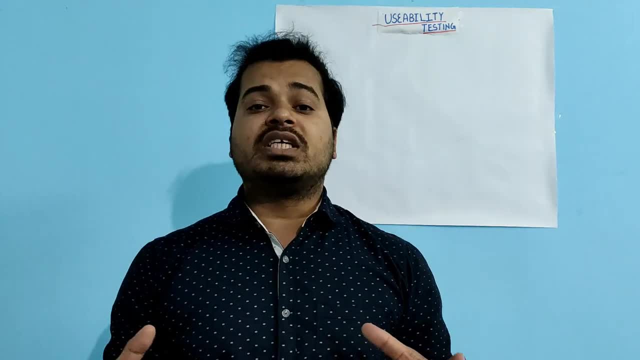 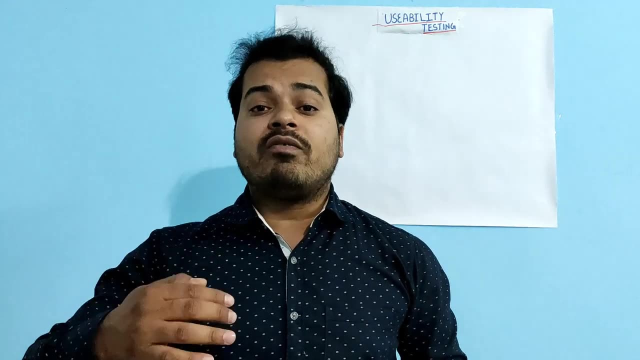 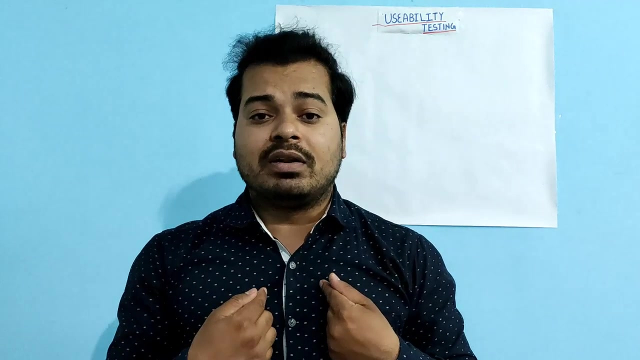 Guys, as you know, when any company is developing the software, they will develop by how they use it. They want it, but we always have to develop any software thinking in mind that this software is not going to be used by our people. 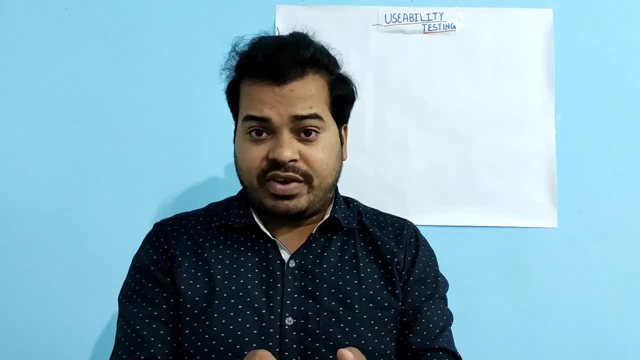 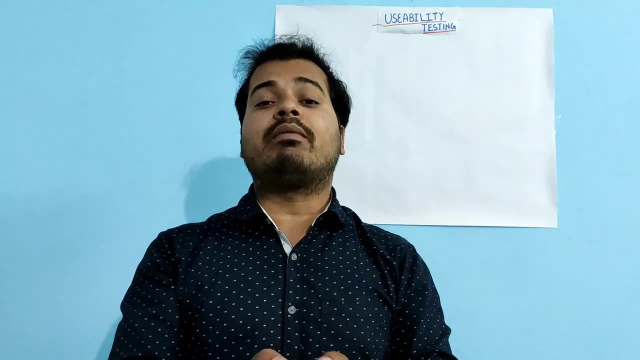 Or I am not the only person who is going to use that particular software, Or whoever is working in this company will not use that software. We have to think that this particular software can be used by anyone, so that it should be user-friendly, so that people can use it. 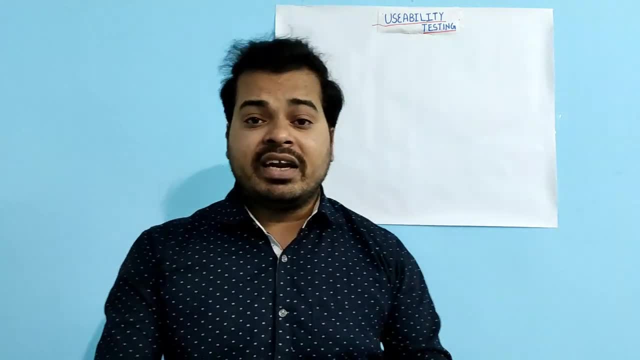 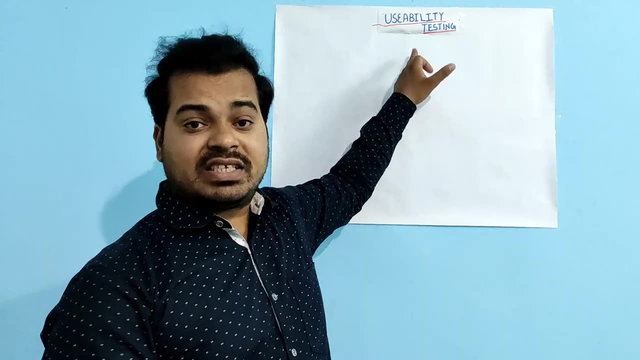 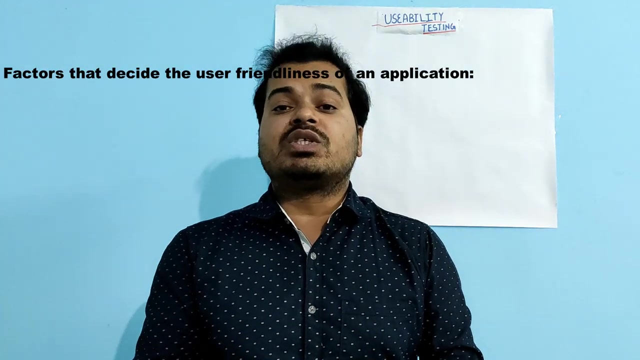 That is called as usability testing. Here we make sure that my application is very user-friendly. It is called as usability testing. So now the question arises on what factors you decide whether your application is user-friendly or not. First one: it should be easily accessible. 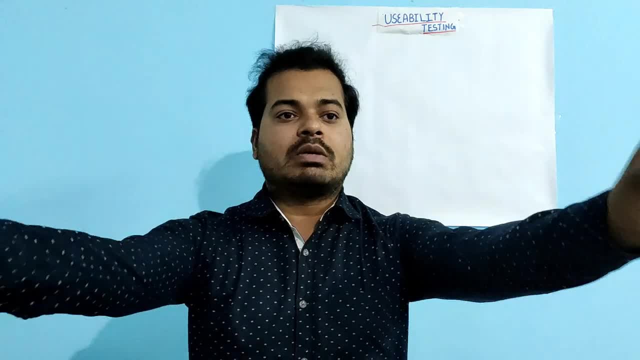 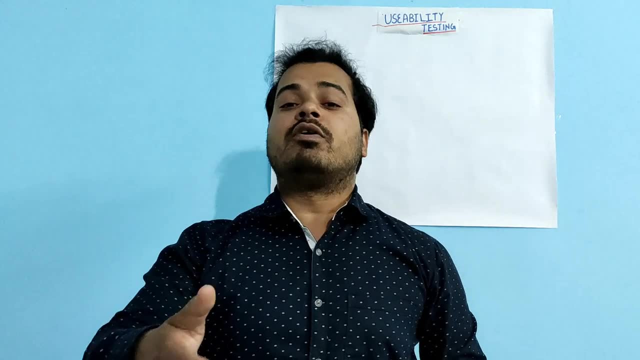 First of all, it should be easily accessible. Now suppose you are launching any company. Let's suppose you are launching a company named as abccom And you have a particular software Which performs something. Now you cannot expect people to come to your website like abccom. 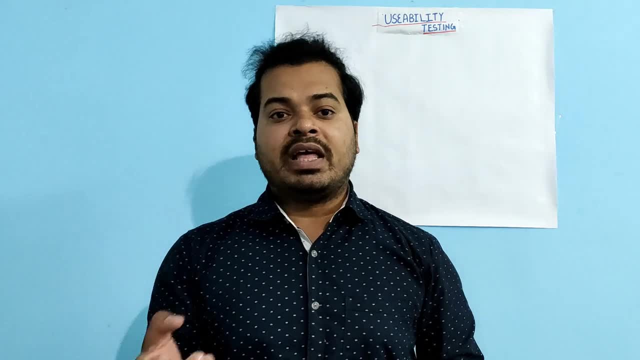 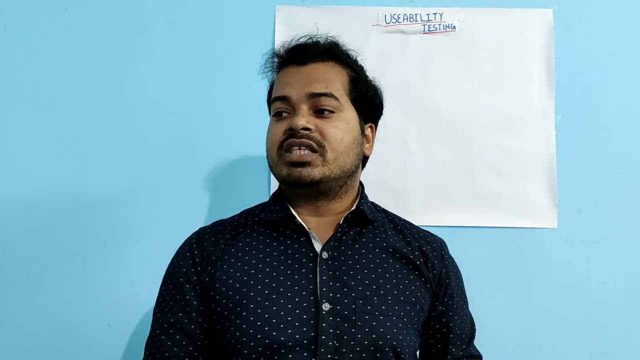 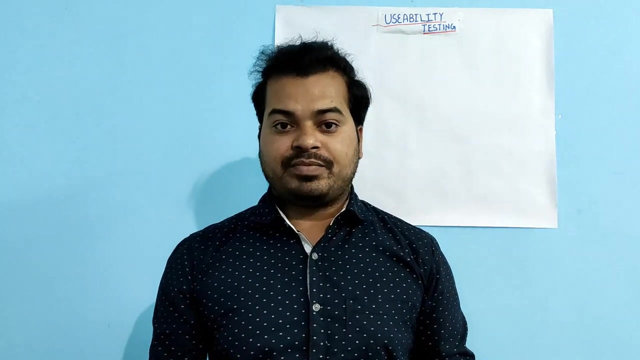 Opening their browser and entering abccom And they are going to download your particular software And they will install in your mobile. This is not user-friendly. If you say easily accessible, that means every application in today's generation is available on the play store or on the ios store. 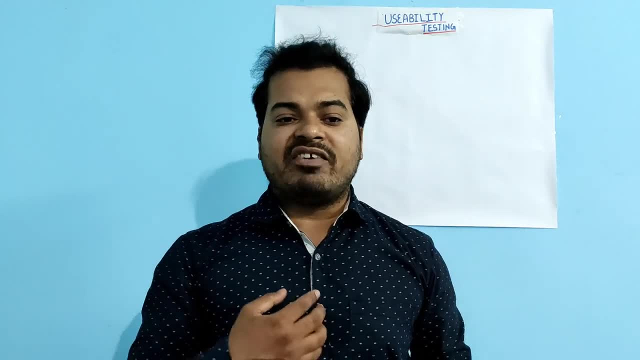 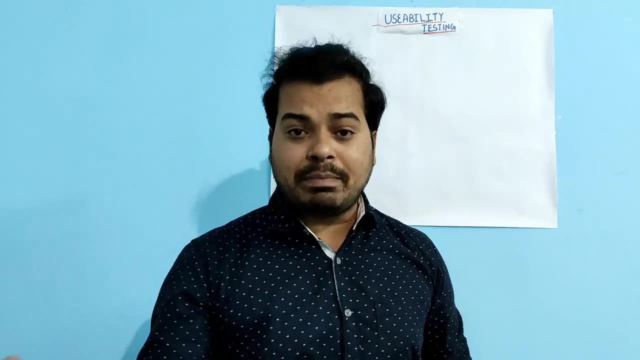 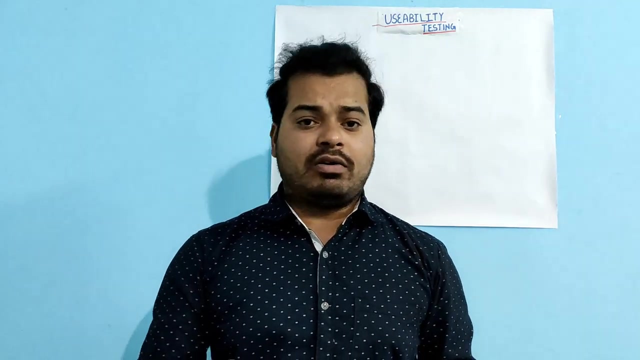 So we have to make sure that if we are launching any application And we want that particular application to be easily accessible to the people, We have to make sure that we will make it available on the google store or ios store Or somewhere where people can go and download it very easily. 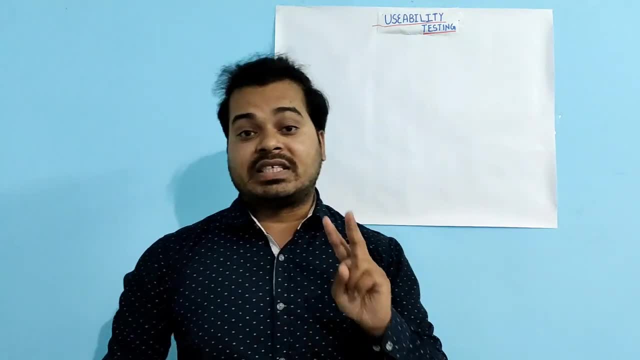 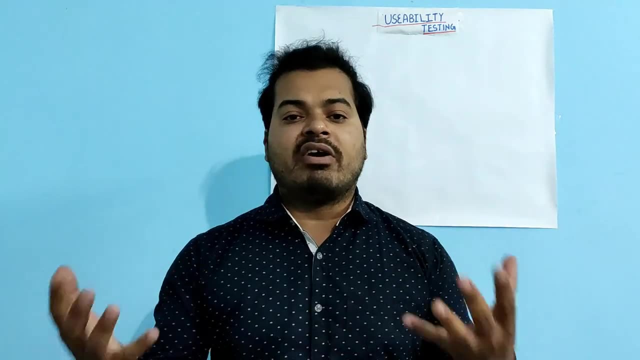 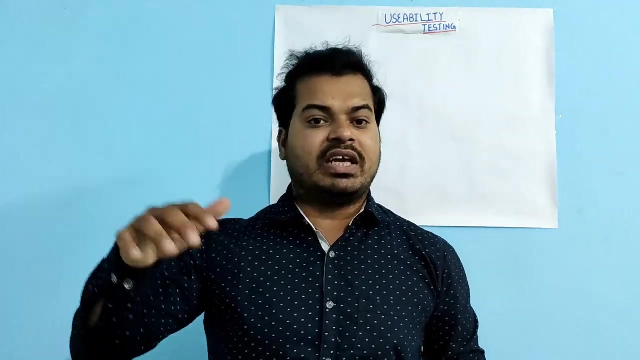 That is called as easily accessible. Second point: your application should be in a very easy language. Whatever the application you have developed, Whichever component is there, Whichever English words you are using Or whichever words you are using, In whichever language you are using, 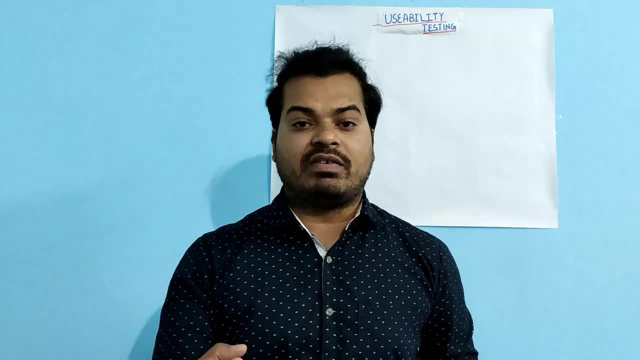 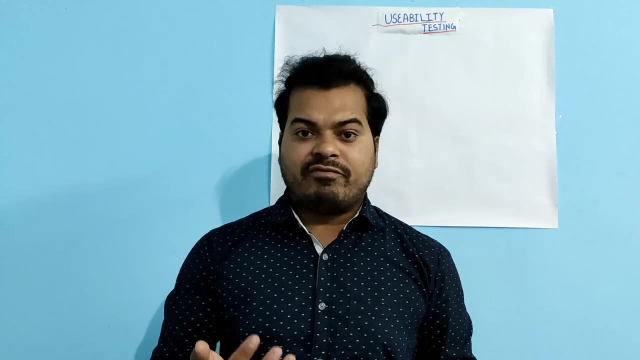 Whatever the words you are using should be in a very easy language. It should not be tough words. Suppose you are using any component. Whatever the name you are giving Like, if you talk about any registration page, It will be having first name, last name, contact number. 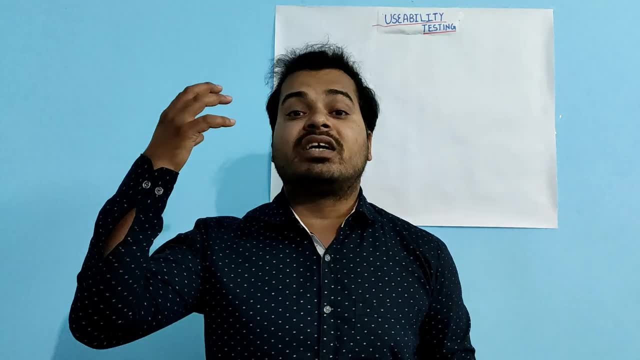 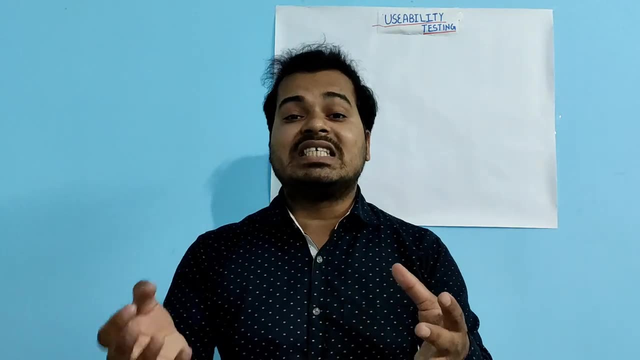 These are not. terms are very easy. You cannot give any hard term, Which is not like. People should not feel that, oh, what is that? And they should go and finally google. it Should be very easy. It should be very easy language. 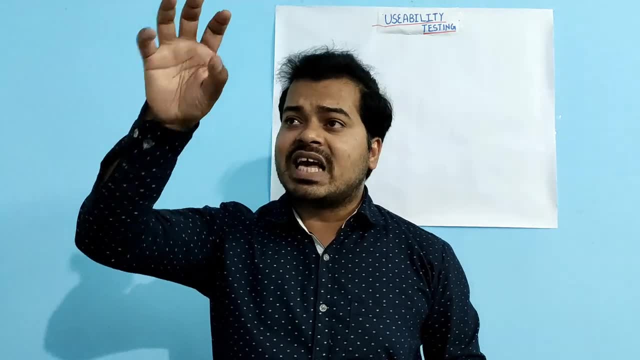 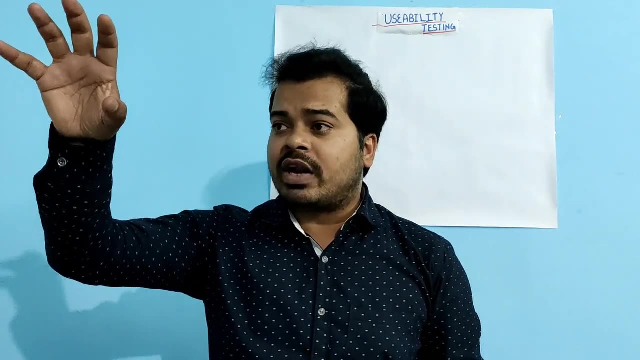 Throughout the application, Wherever you are using any word, Whichever language you are using. I am talking about language English. If you are using your application totally in English, All the words you are using in any component Or you are giving. 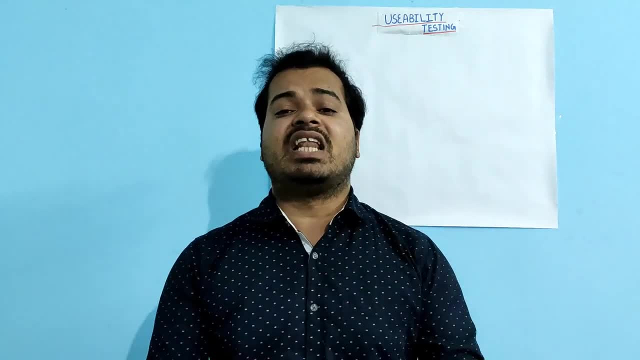 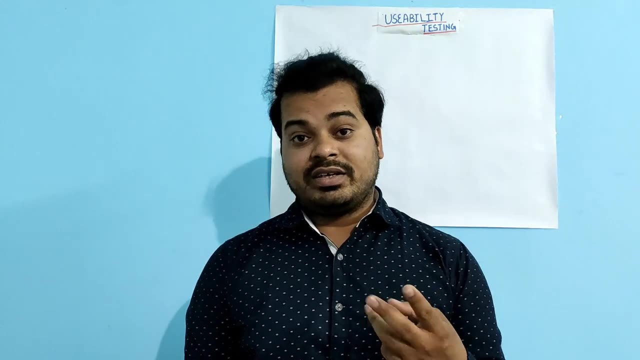 Whatever you are doing, It should be in a very easy language. It should be understandable by anyone in this world. It should be understandable by the person who is using it. Third is called, as It should be easy to understand, Whatever the application you have developed. 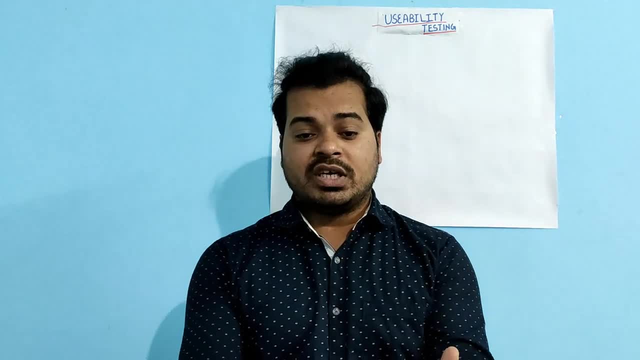 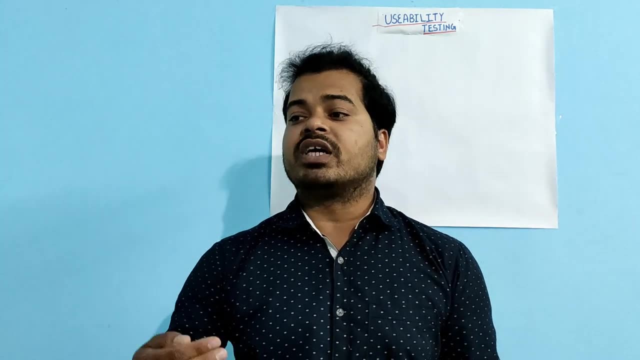 And, finally, you are giving it to the customer to use it. The application should be very understandable So that if people are not able to understand, If your consumer, If your customer are not able to understand, What is the use of this application. 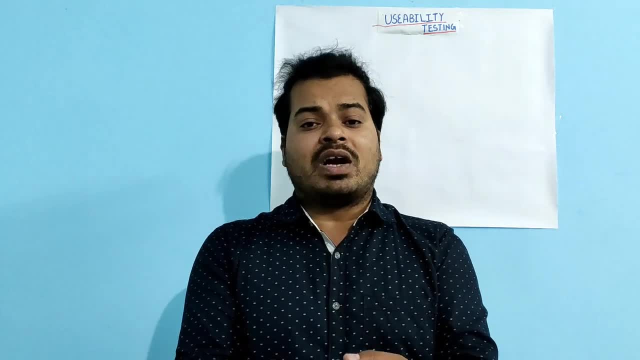 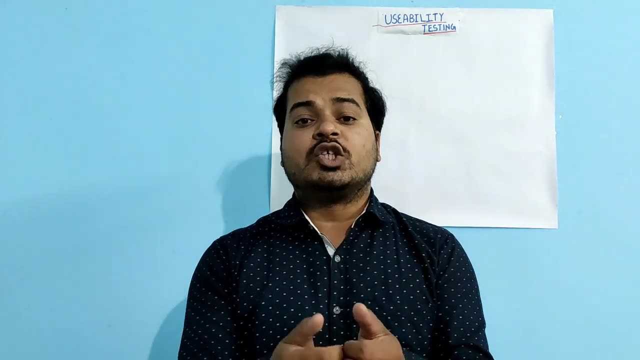 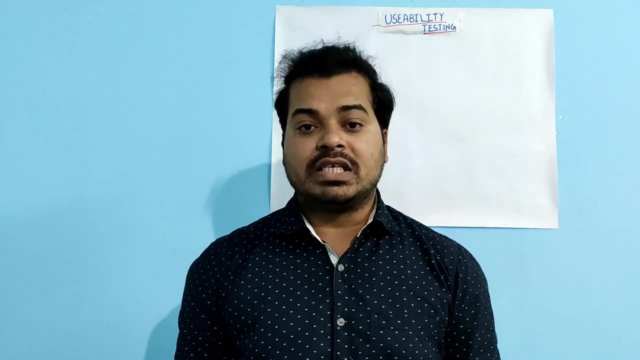 What it does. If people are not able to understand What you have developed, It is of no use. So whatever the application you are developing Should be easily understandable by the people. Fourth point: Proper help text message should be displayed, Suppose: 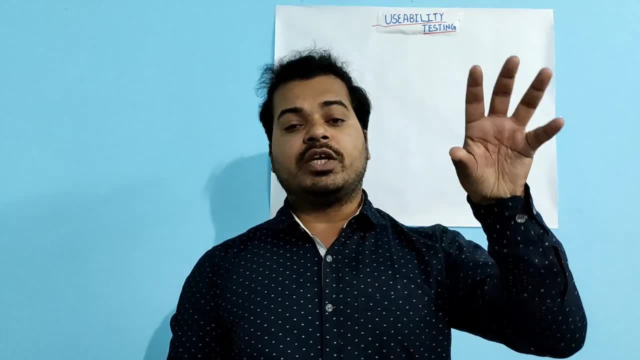 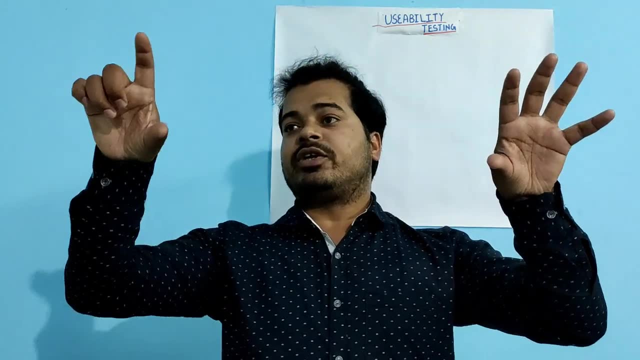 If some application is there Where they are asking you to fill your name, Just name. they have filled Just name, they have told And they have given it to Text field to enter. Now they should give place holder also inside that, Inside that two fields. 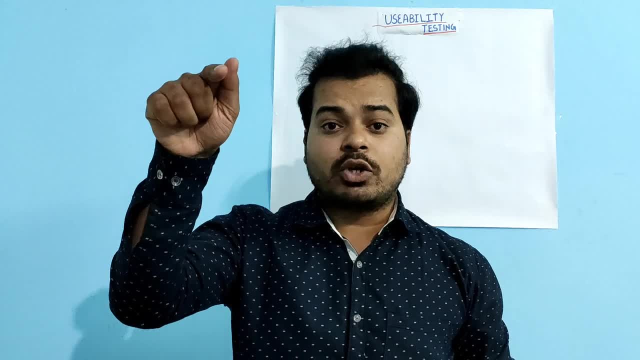 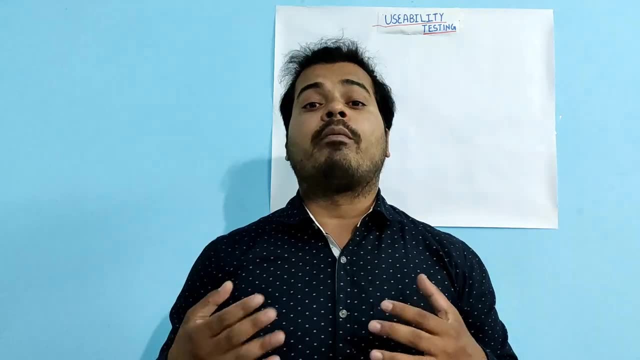 First one is your first name. Inside it place holder should be written Like it is a first name. Inside your second box It should be written as your last name. Proper help text message should be displayed In order to make people understand what they are asking. 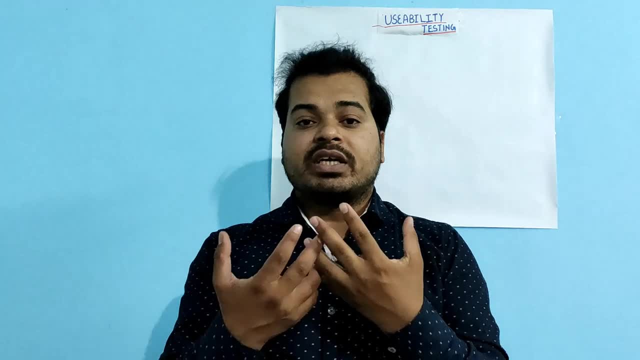 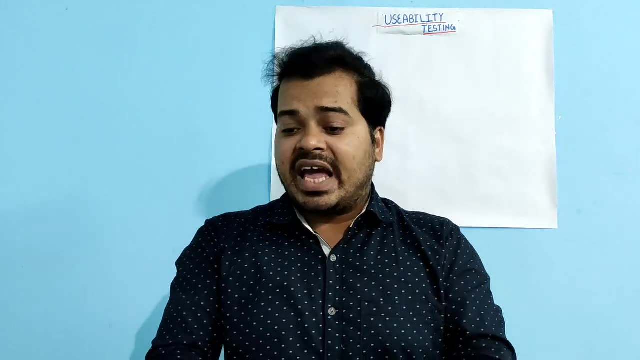 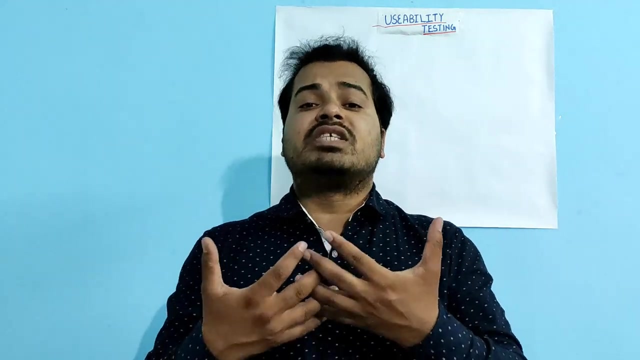 Number five: When people are trying to enter any wrong data Or When people are Enter entering any wrong value In any of the text field Or any text area field Or anywhere in an application. If user is doing some mistake. 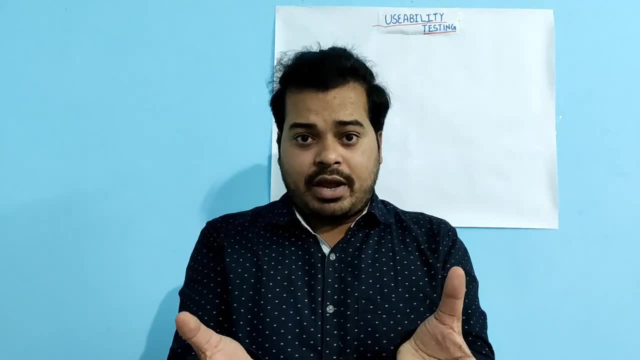 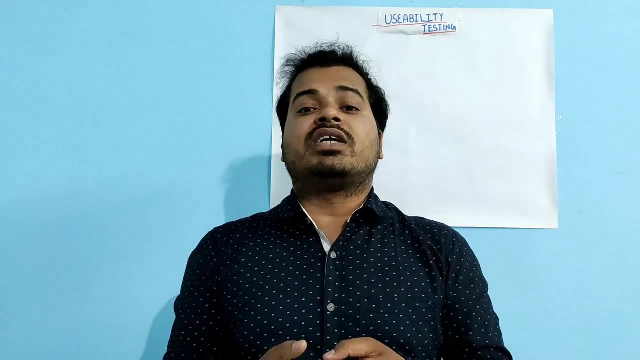 It should throw a pop up saying that You are doing this mistake. Let's say, some text field is there Which can accept only alphabetical characters And you are trying to enter Numeric digits. It should throw an error Or pop up saying that. 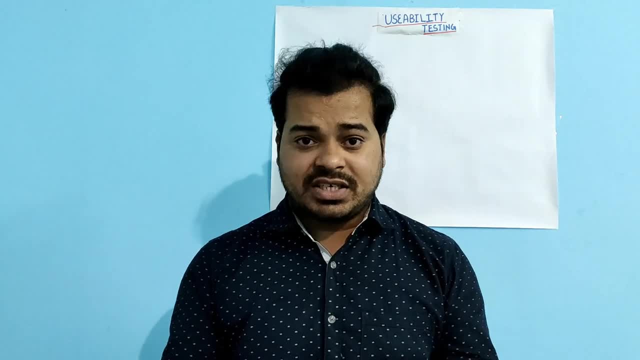 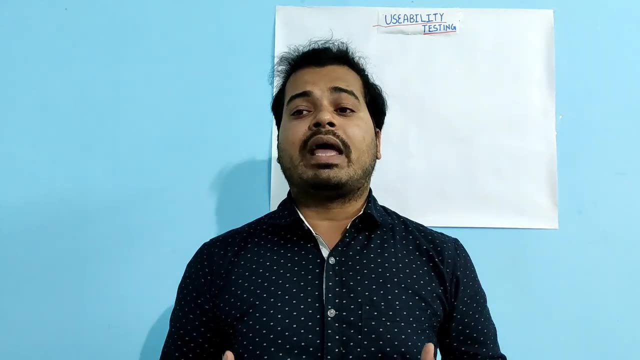 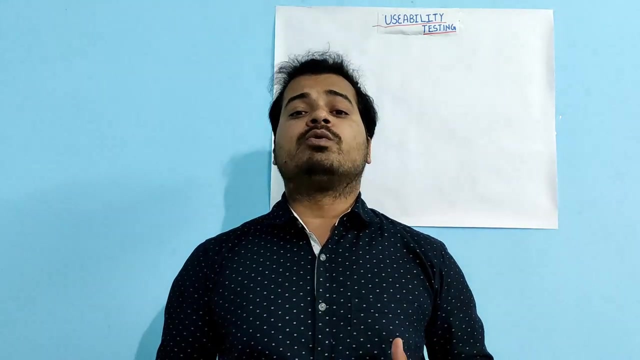 This text field cannot accept Numeric digit. This is called as Throwing an error message And helping people understand What my application do, What my application accepts. Sixth, We have to make sure that My application is very user friendly. 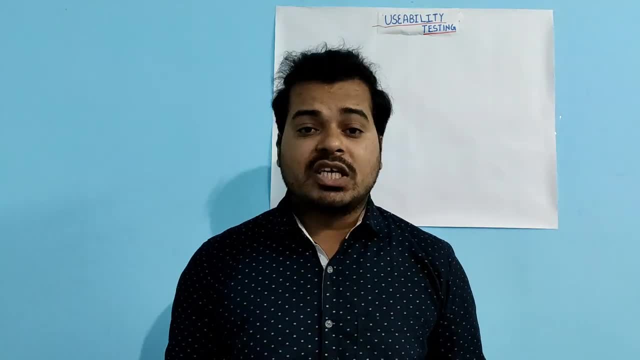 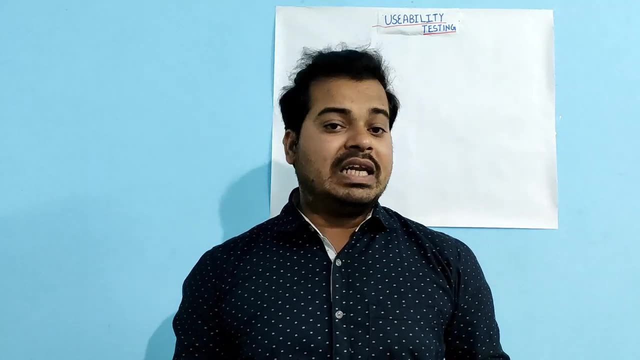 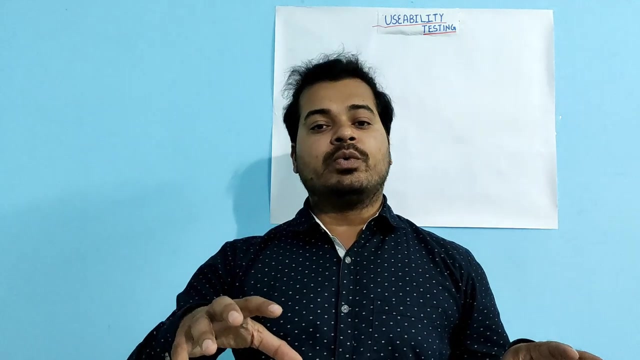 How? Because my application Look and feel of an application is very good. Seventh, Navigation should be very simple. Let's take example of Amazon. You are logging into Amazon website. You are selecting a product, You are adding it to your cart. 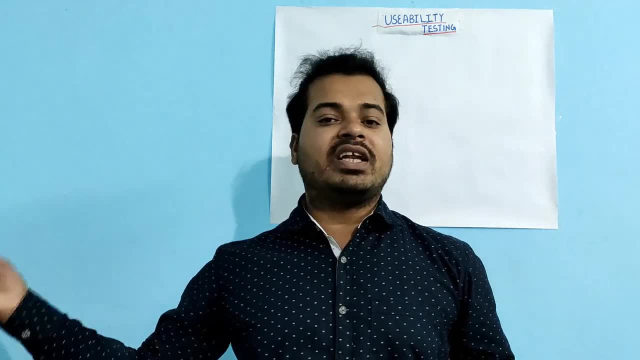 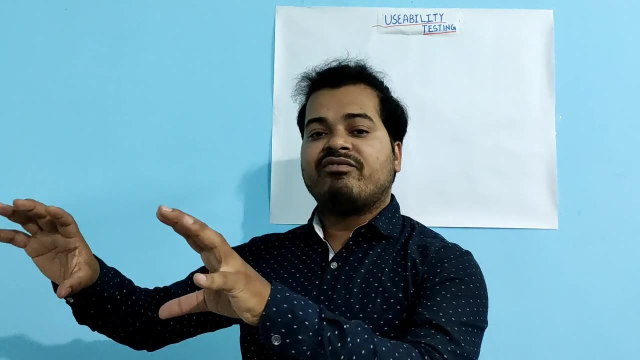 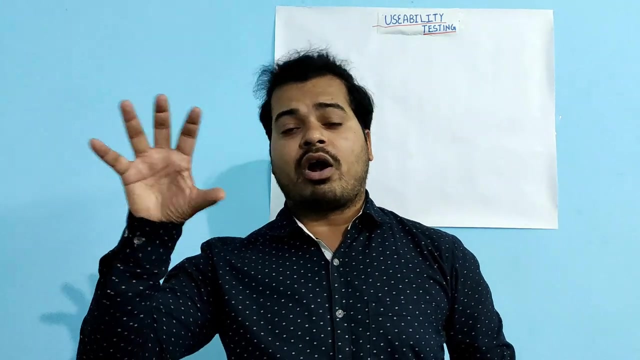 You are doing a payment. Finally, it is showing you that Your order has been placed. That is what I am telling. Navigation to each and every component Or each and every module, Should be very easy, Just giving an example. Suppose you have added your product. 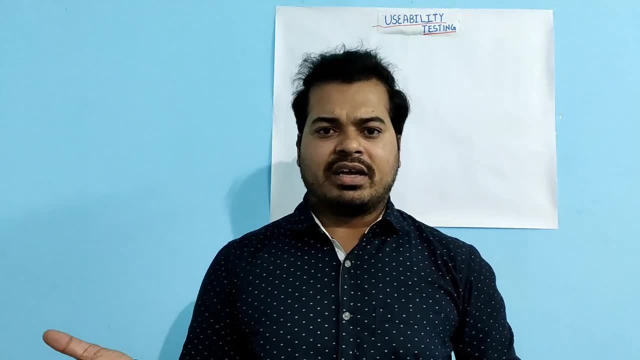 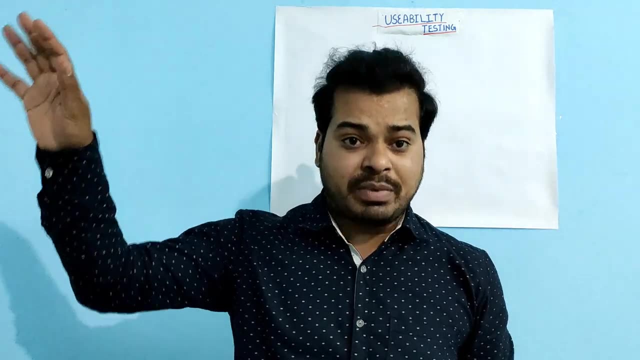 Into your cart And now some other pages are coming Like: select this product also. Select this product also. There is no option to go to the payment page Or there is no option to go to your cart page. I mean people will say